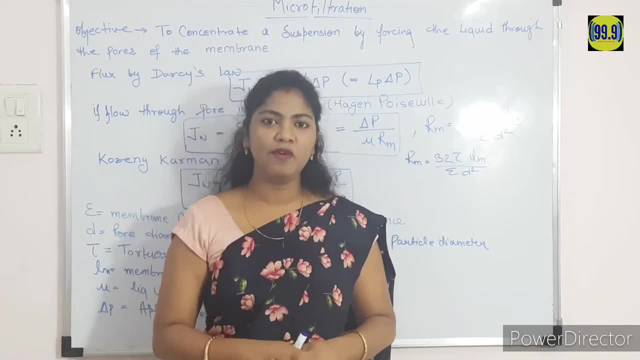 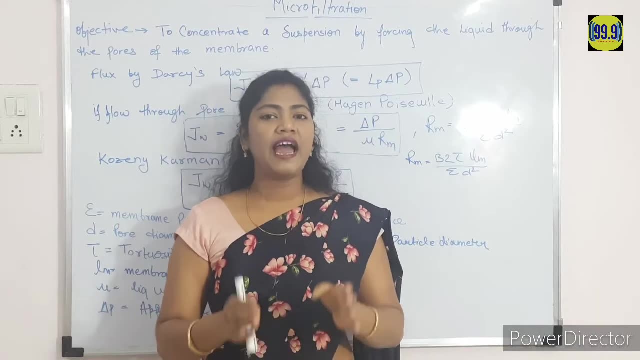 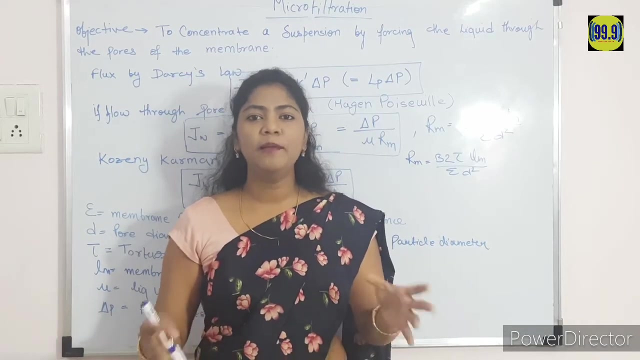 channel. subscribe it, otherwise you will not get any type of notification from my site. And one more important thing is that you have to follow me on telegram, because in telegram I used to post many important questions, numerical pdf, short notes, notes and many more things. So follow me there and subscribe my youtube channel. So, without further ado, let's. 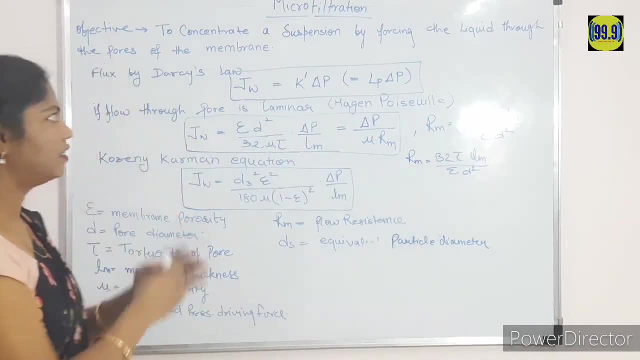 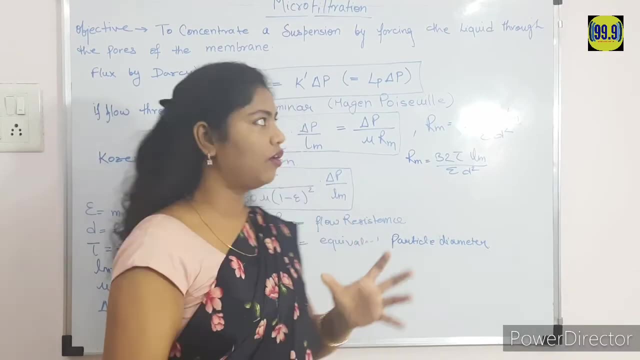 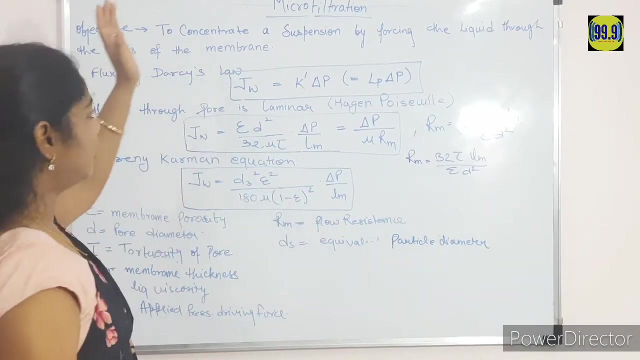 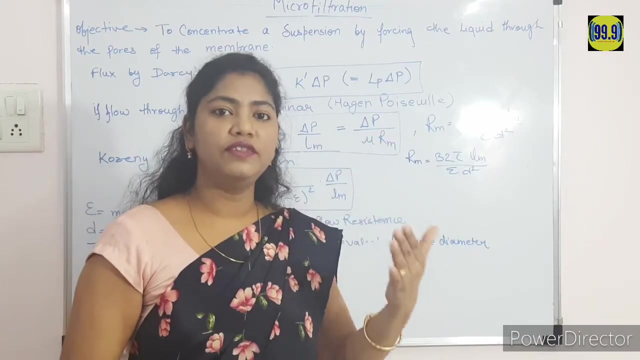 get started with the lecture and the topic. So, as we know that the micro filtration play a very important role in the membrane separation operation. Okay, so the if we discuss the objective of the micro filtration, That is, to concentrate the suspension by forcing the liquid through the pores of the membrane. 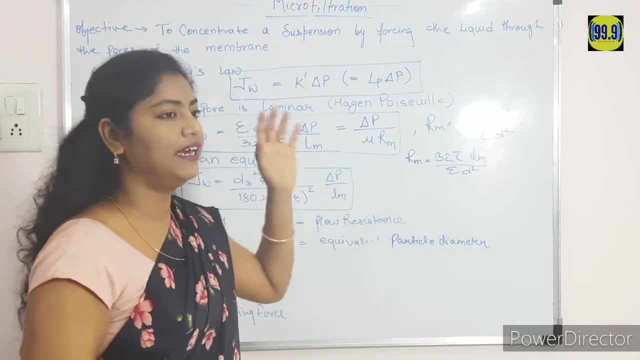 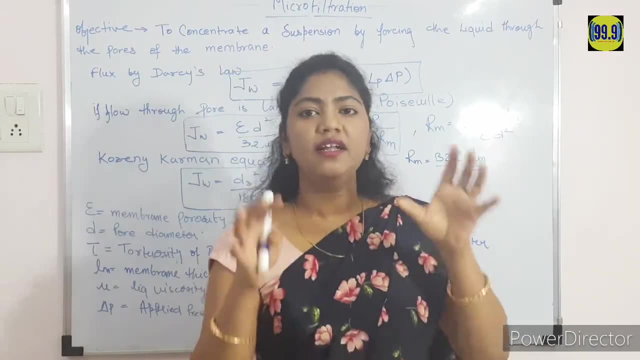 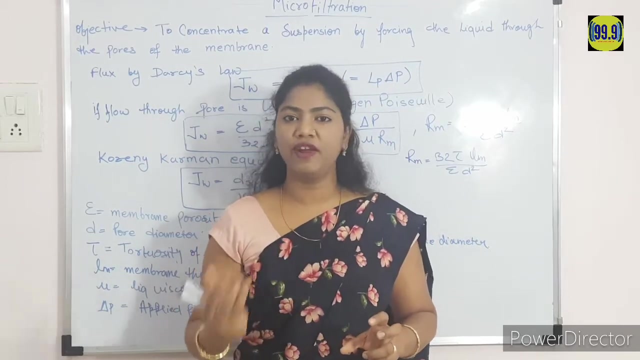 It means we have to force the suspended concentrated liquid through the pores of the membrane. Okay, so this is the objective. So we have to calculate. the main thing is that we have to calculate the solvent flux. Okay, we have to calculate the solvent flux and how we calculate. 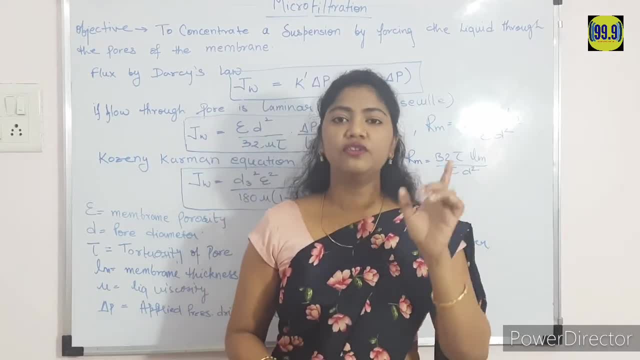 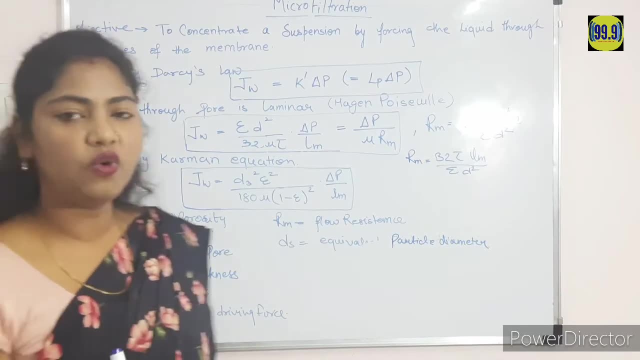 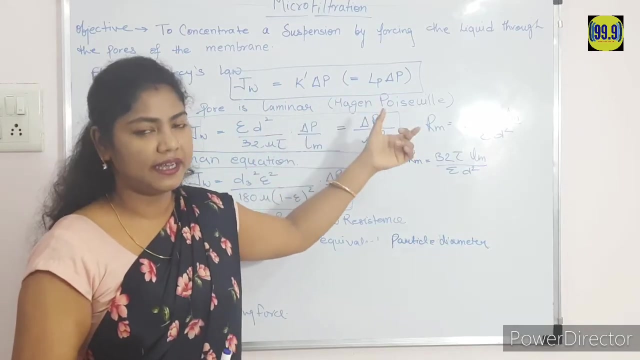 the solvent flux By using the number of equation. So the first one is the by Darcy equation. So let's discuss the Darcy equation. that is equal to: jw is equal to k dash delta p. jw is equal to k dash delta p. 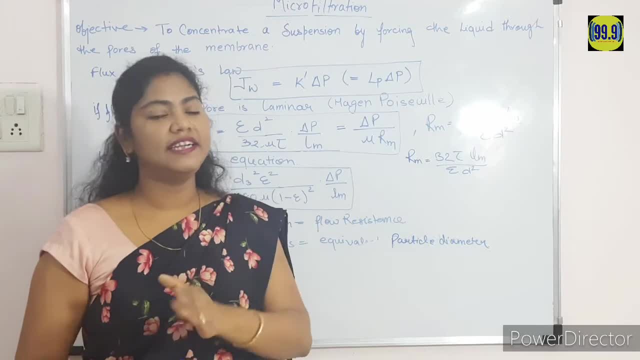 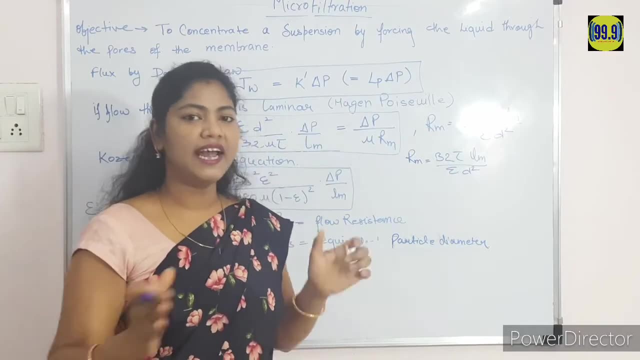 Or you can also write it as lp, delta p, Okay, so here delta p is the applied pressure driving force and k is the constant. Okay, k is the constant. Okay, so here delta p is the applied pressure driving force and k is the constant, Which is same as the water permeability. 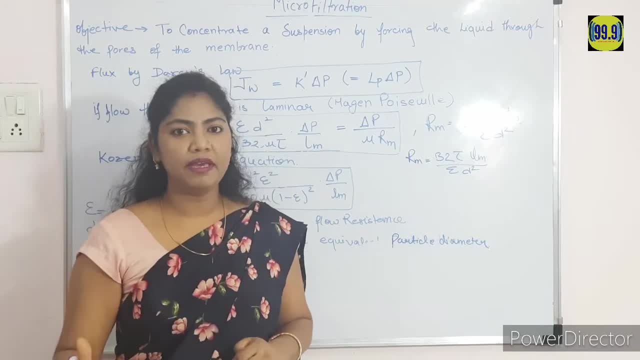 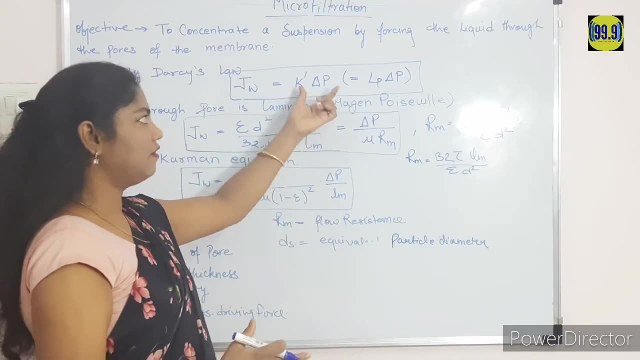 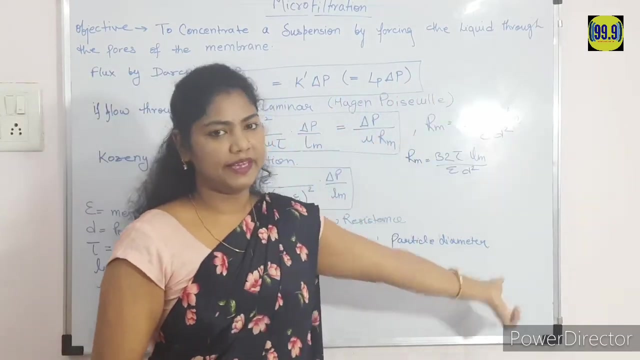 Which is same as the water permeability, Which is same as the water permeability lp. Water permeability is represented by the lp. That's why we replace this equation- or you can also write this equation as: jw is equal to lp, delta p- okay, And its value depends upon on difference value of the membrane parameters. 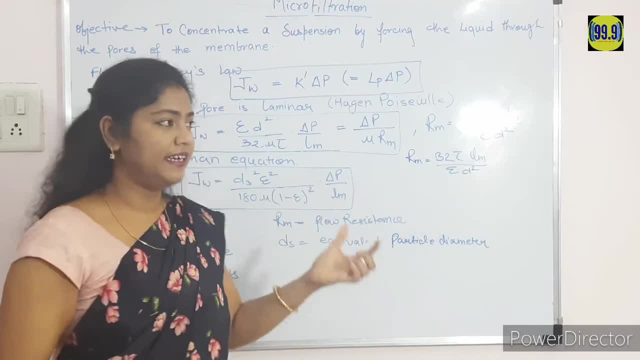 Okay, and its value depends upon on the difference value of the membrane parameters like porosity to setzt detail system Н and T: Okay. so in theseaufcase the softener is equal to very, to the forme: Okay, And at least one strand we have to regulate. 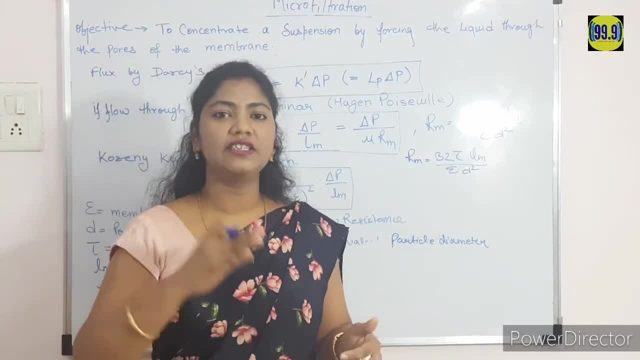 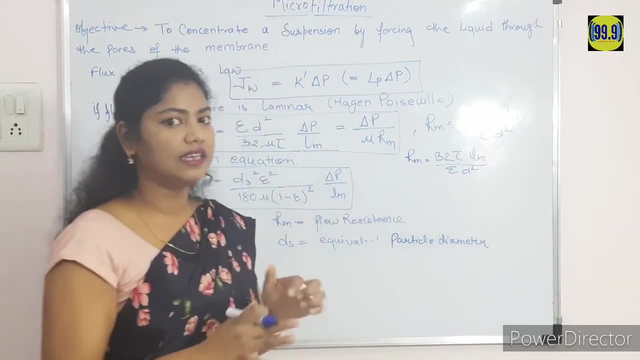 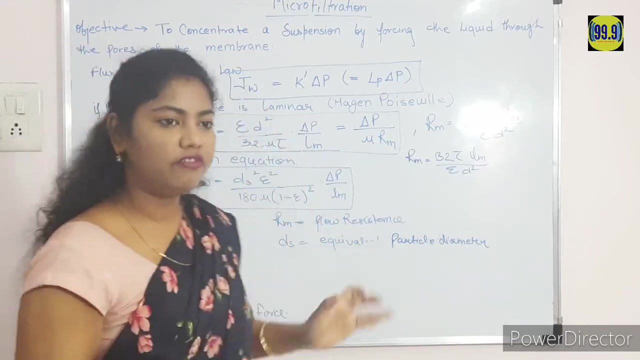 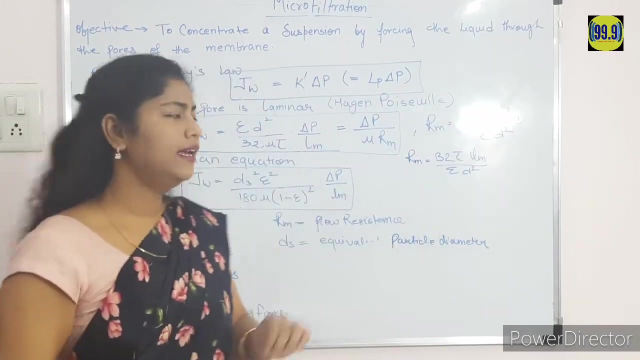 like porosity, torticity, pore size, distribution, liquid density, viscosity- all these are depends upon these parameters. okay, So formula which is used for calculating the solvent flux by the Darcy equation is: Jw is equal to Lp, delta p. okay, that's it. okay, Now what happens if the flow in 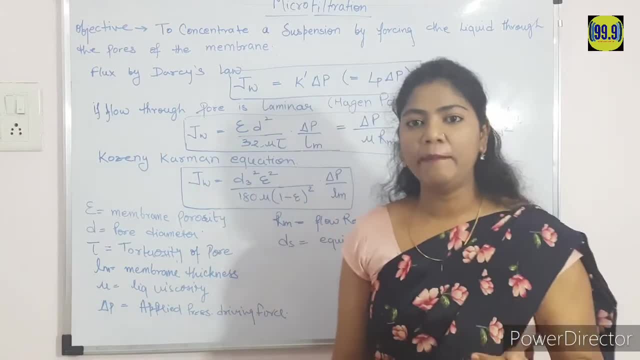 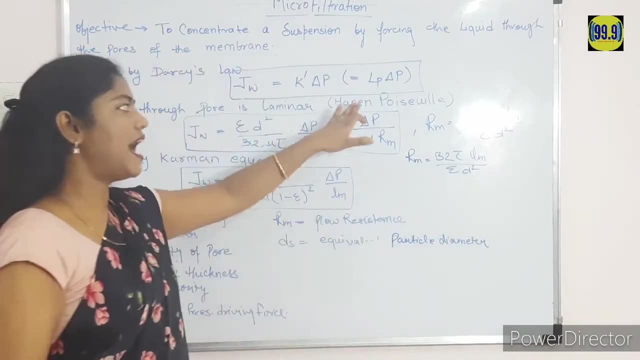 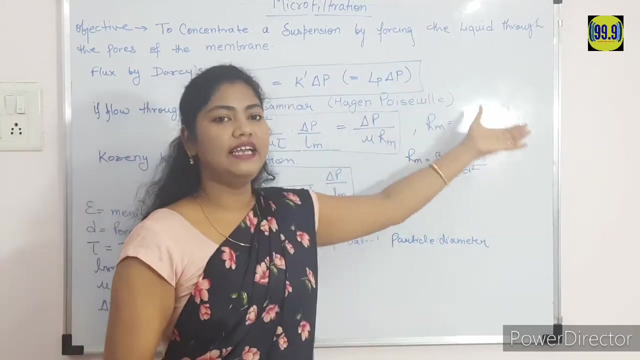 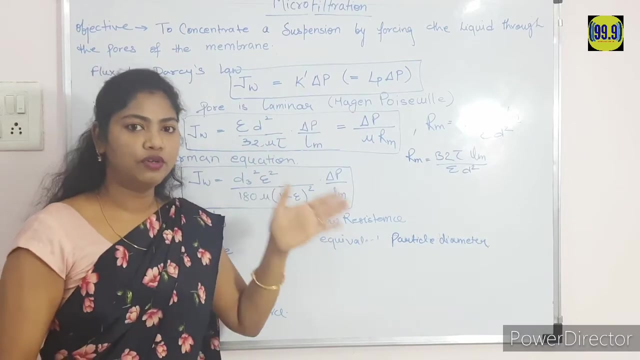 the pore is laminar, then what will happen and which type of equation we can use where that for calculating the solvent pores is the Heisen-Posley equation. We calculate the solvent flux by the Heisen-Posley equation, and that is, that is equal to sigma d square upon 32 mu tor. 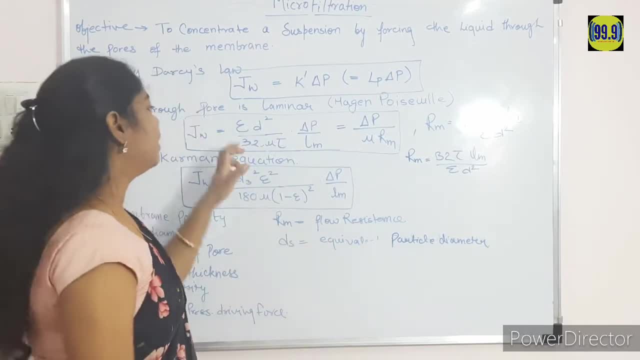 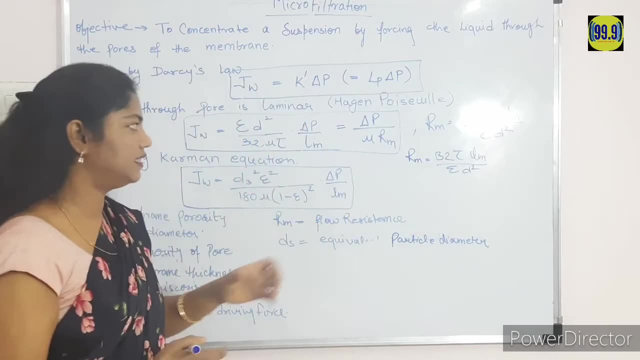 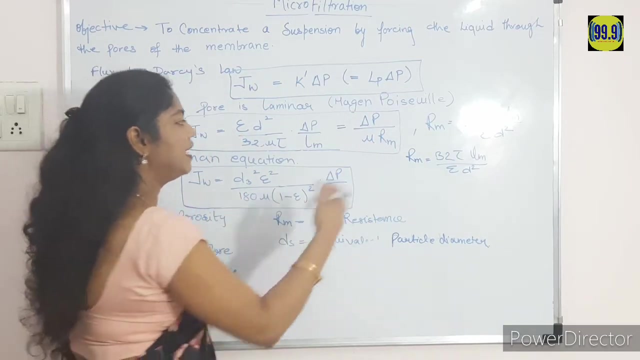 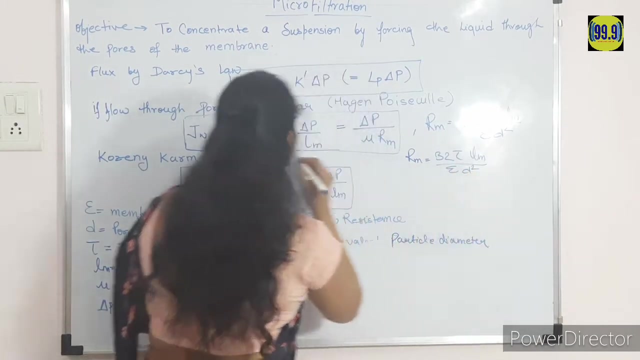 into delta p upon Lm. okay, and we can also replace this equation, some constant, by the resistance, flow resistance, and we can write it as a delta p, mu, Rm. it means we replace which parameters? we replace Rm by 32 tor, lm by sigma d square. we. 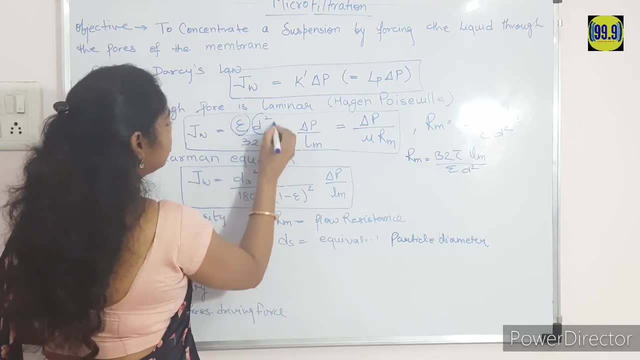 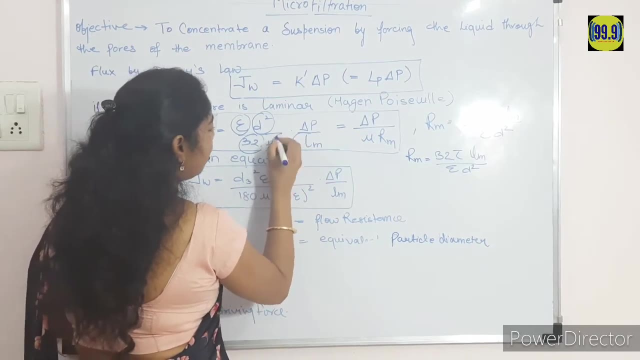 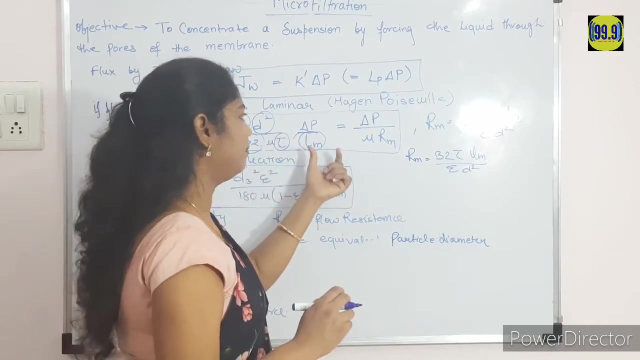 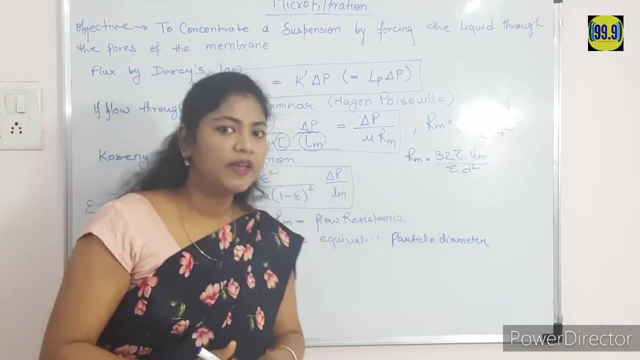 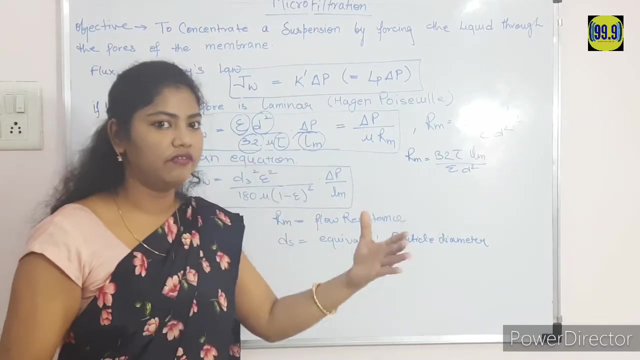 replace sigma d square 32, mu or and mu. sorry, minwe, not mu- tor, lm, over Lm and lm. we replace it by rm, we give them a name, rm, and we reduce this equation into a. jw is equal to delta p, mu, rm. okay, that's it. so we can. if the flow is laminar, we use to calculate the solvent. 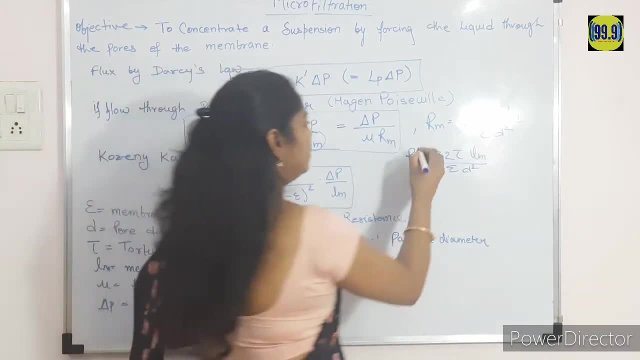 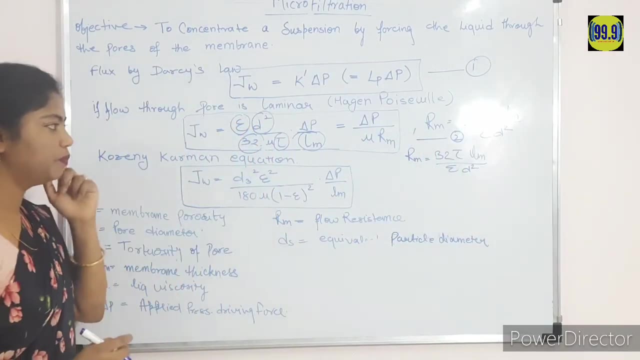 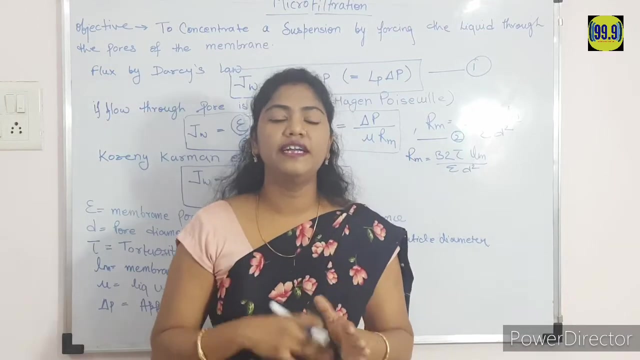 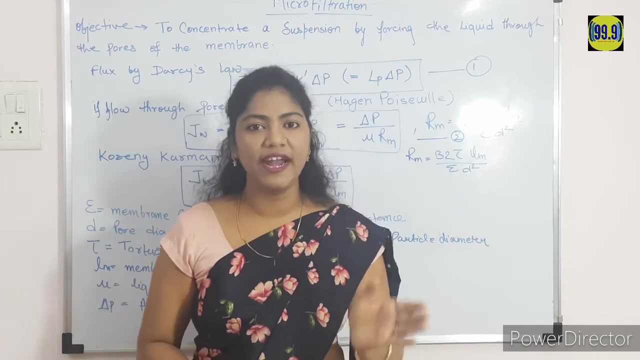 flux, with this equation, which is equation number two, we consider. this one is the equation number one, and this one is the equation number two. now, now, the another important thing is that what will happen, or what type of flux we use for calculating when the membrane contains some type of void. 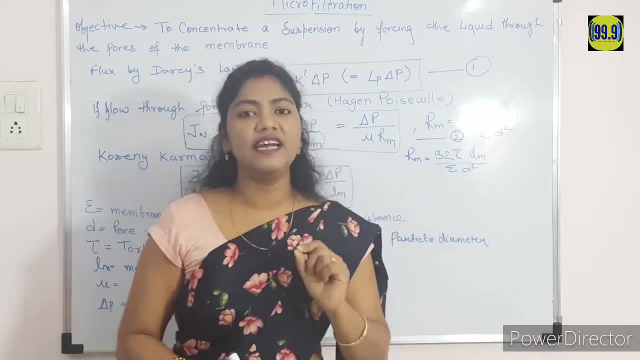 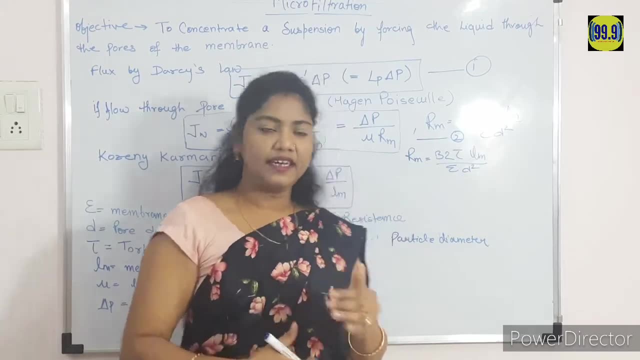 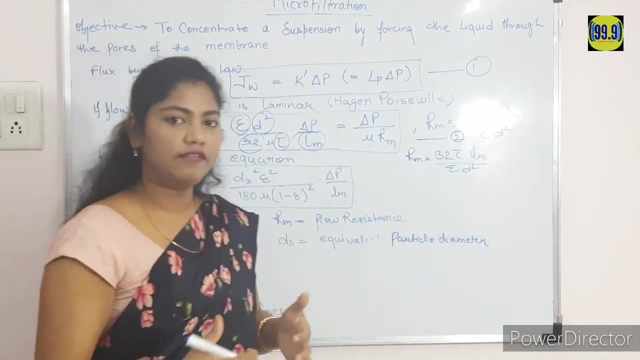 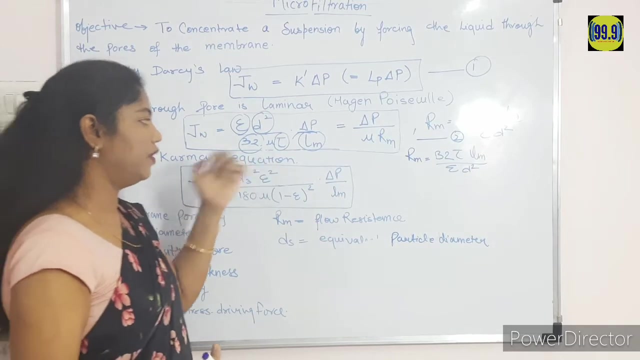 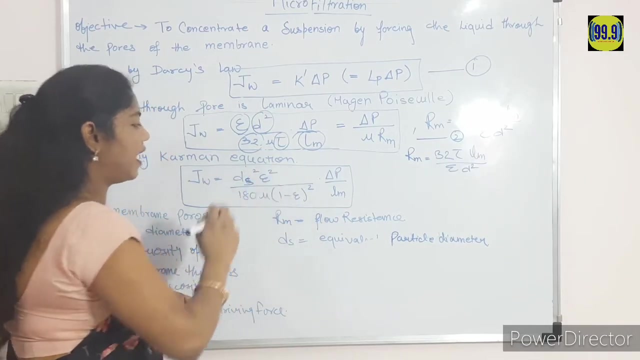 spaces, then in that case we consider it as a peg bed. in that case we consider it as a peg bed and in that case we solve or we calculate the jw, that is solvent flux, with a formula, or we can form formula by cosin carman equation by what was that? that is, jw is equal to ds square, square, sigma square. 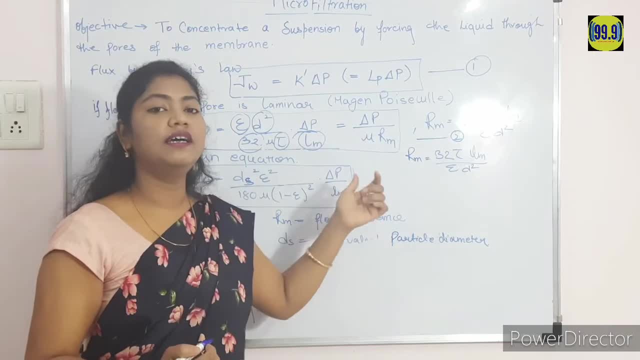 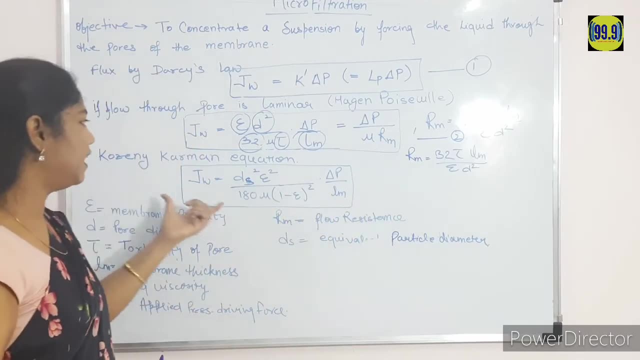 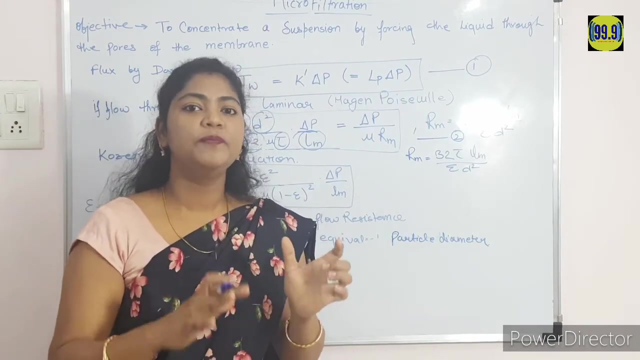 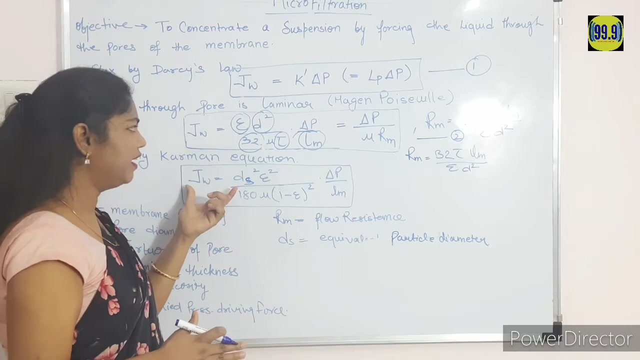 upon 180 mu, 1 minus sigma to power to whole, 1 minus sigma to power, square delta, p upon lm. so this is the equation. when we consider the void spaces and we can say that the membrane is behave like a peg bed, then only we use this type of equation. now discuss the. what are the parameter notifications that? 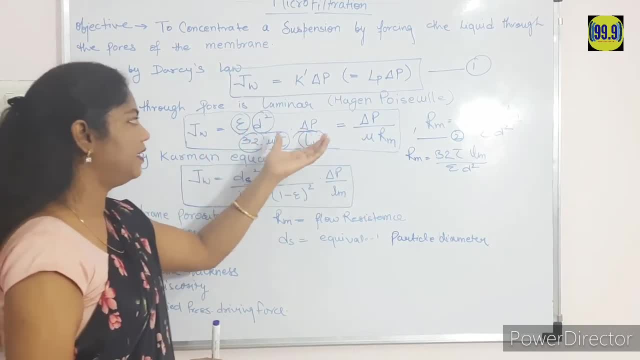 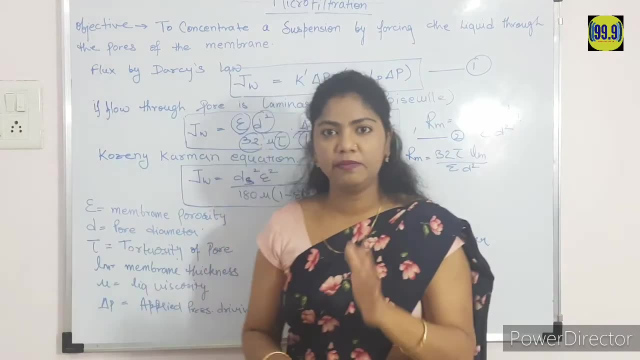 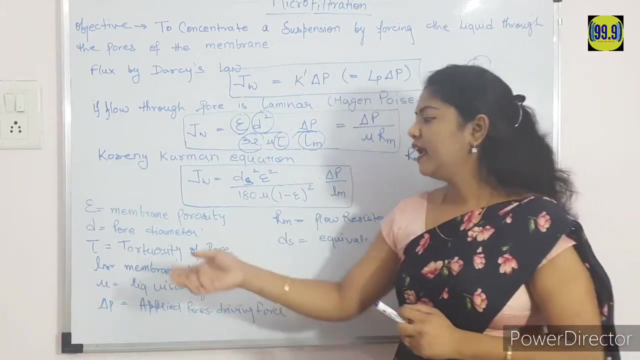 how we can identify the which parameter will indicate what thing. so the here, the sigma, represent the membrane porosity. sigma is basically the membrane porosity and sigma is the membrane porosity. d is the pore diameter, t is the tortuosity of the pore and lm is the membrane thickness. and 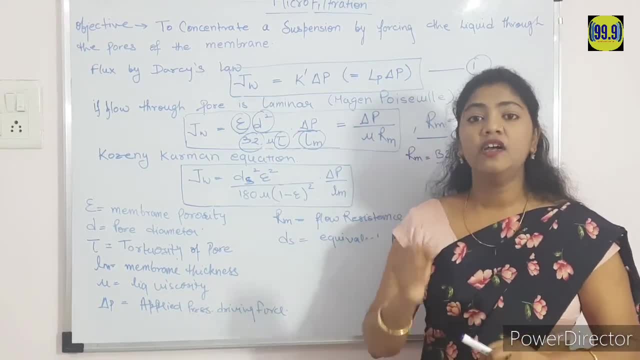 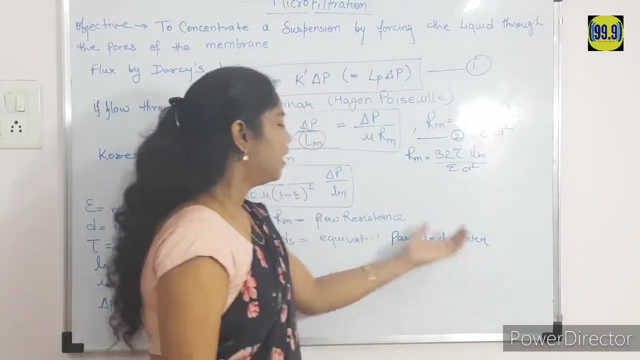 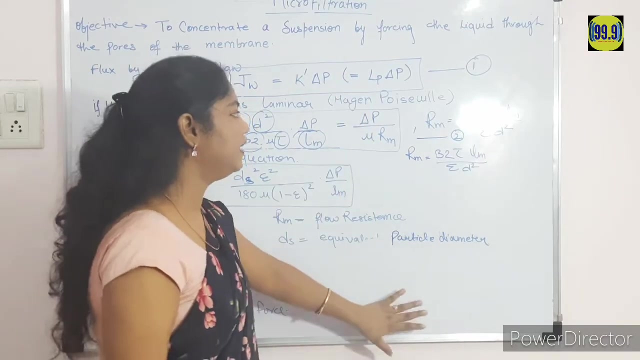 mu is the liquid viscosity and liquid viscosity and delta p is the applied pressure driving force and rm is the rm is the flow resistance, okay, and ds is the equivalent particle diameter. so this is all about the all the formulae. so this is the formulae. so this is the formulae for the flow. 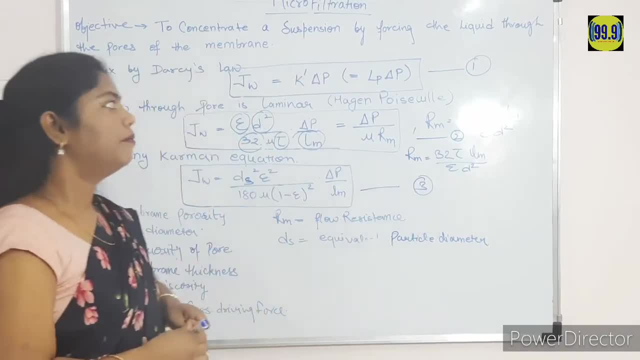 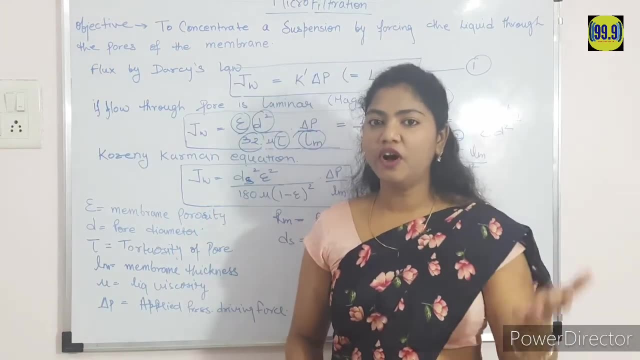 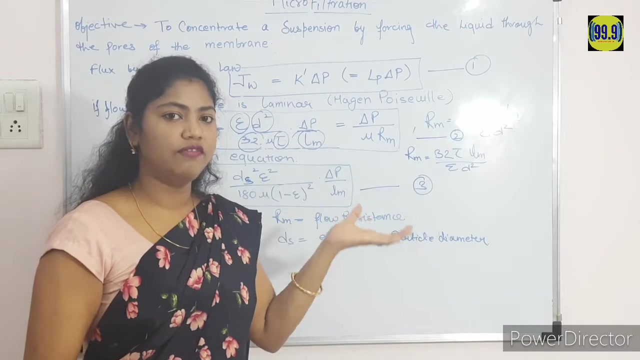 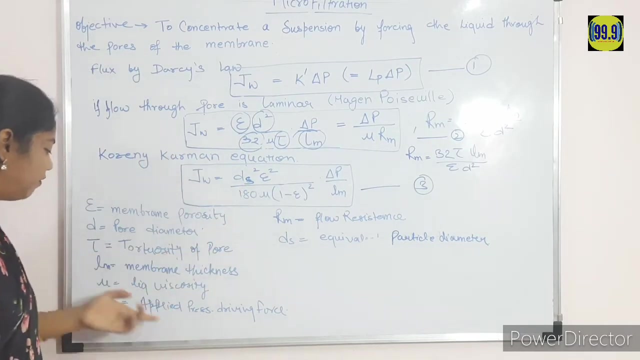 of for calculating the solvent flux based upon the given condition. you can apply this equation and solve it by once. you can solve the various thing from this equation, like you can calculate the liquid of solvent flux, or you can also calculate the resistance, and. or you can also calculate from this equation by. 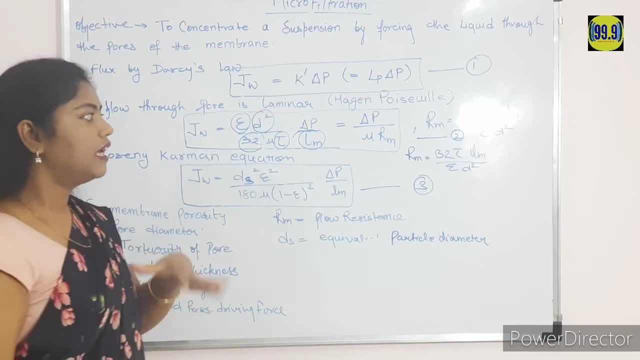 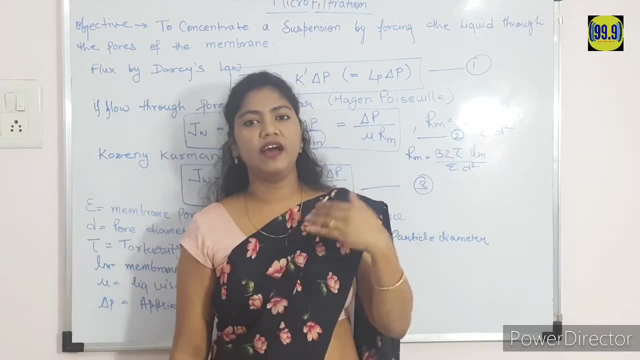 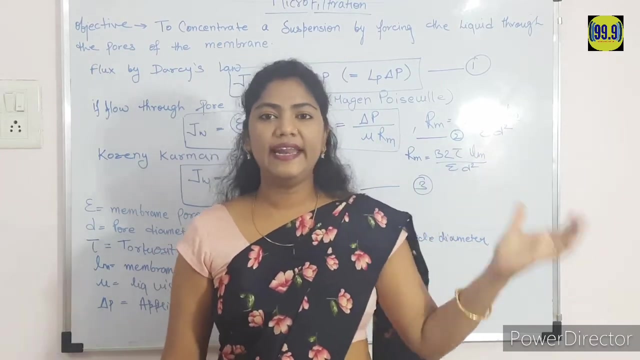 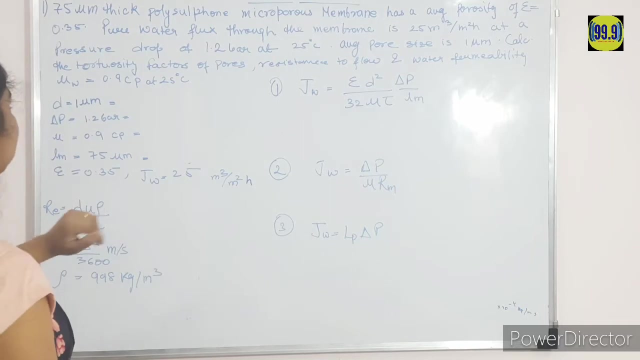 membrane thickness or viscosity if the given condition is asking upon that condition. okay, so now we are going to move to solve some numerical, one numerical which is based upon these equations. so let's get start. so let's discuss the numerical first. okay, so the statement for the numerical is 75. 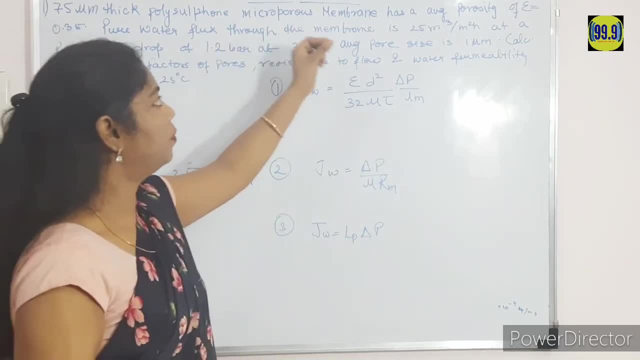 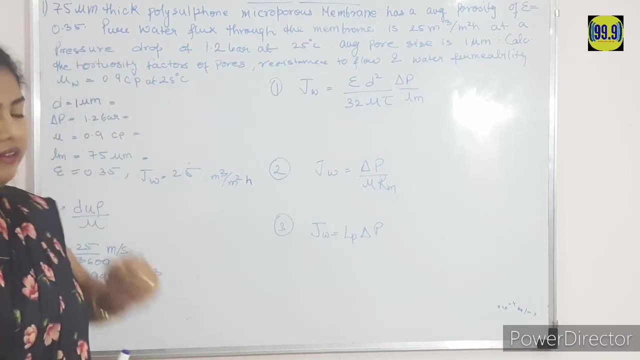 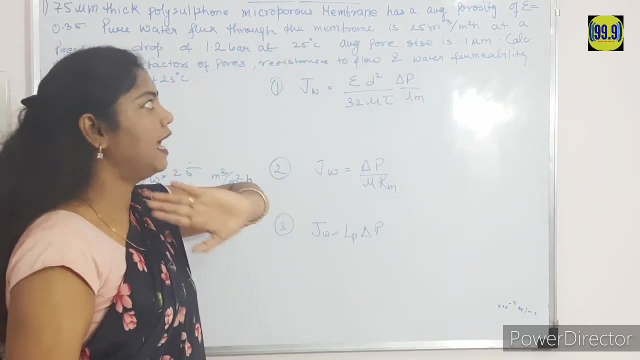 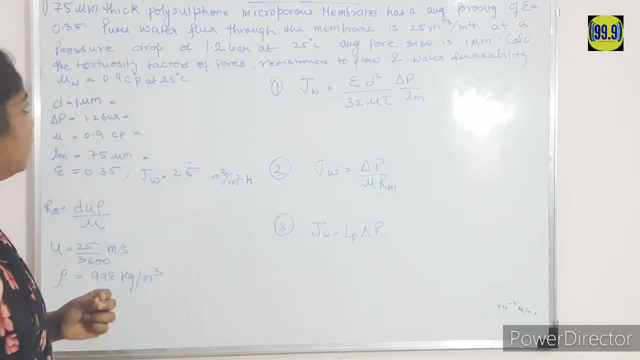 micrometer takes polysulfone micro porous membrane has up, any average porosity of Sigma is equal to 0.35. we have a micro micro filtration, that is polysulfone micro porous membrane, and its average porosity is given in constant. terms of constant, that is 0.35. okay, so the pure 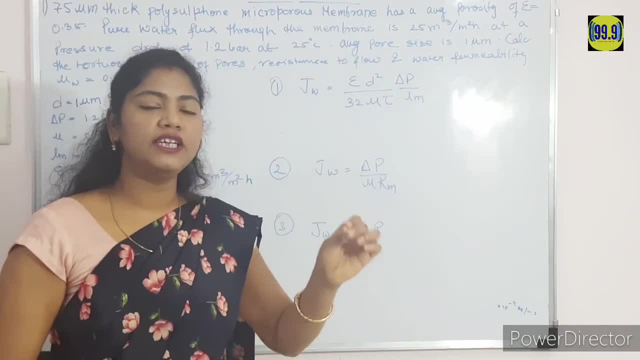 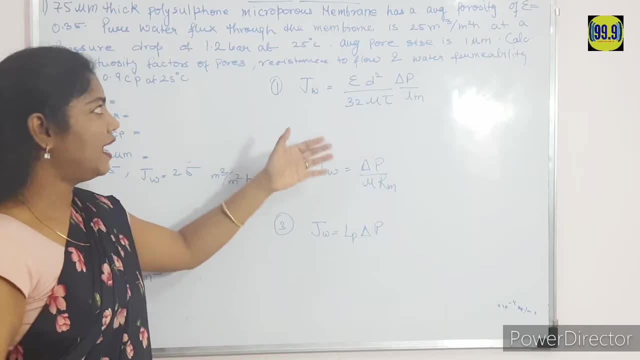 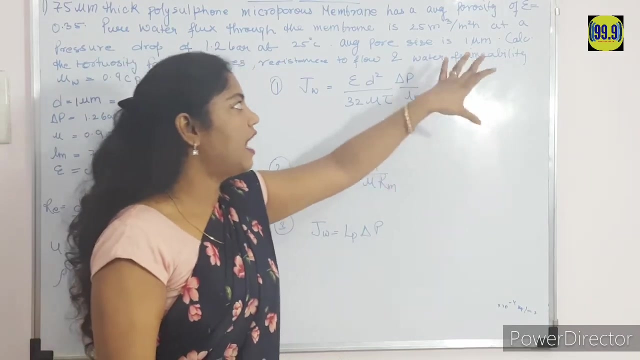 water flux through the membrane is 75 meter cube per meter square are at a pressure drop of 1.35, two bar at 25 degrees Celsius. okay, so the average pore size is, given that, my one micrometer and we have to calculate the toticity factors of the pour. 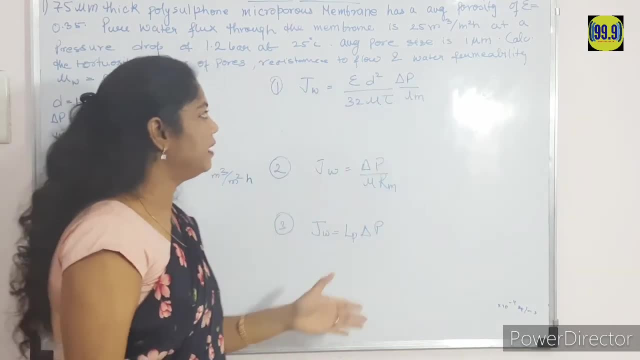 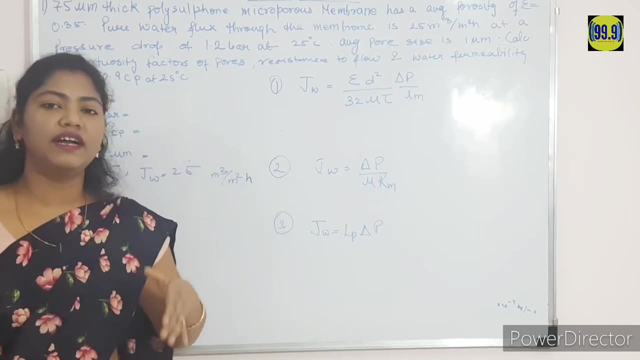 resistance to flow and the water permeability and the given data also. we have that viscosity of water at a given at a 25 degree Celsius is 0.9 CP. so we have to find out three things to calculate for that same as the given ligand, we select the Cpic imgम and the given data also. we have that the viiscosity of water at a given at a 25 degree Celsius is 0.9 cp. so we have to find out three things. 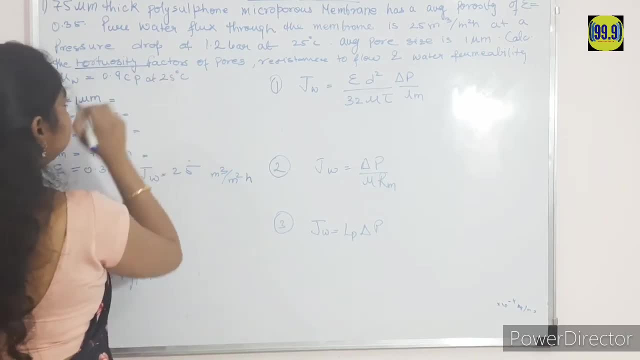 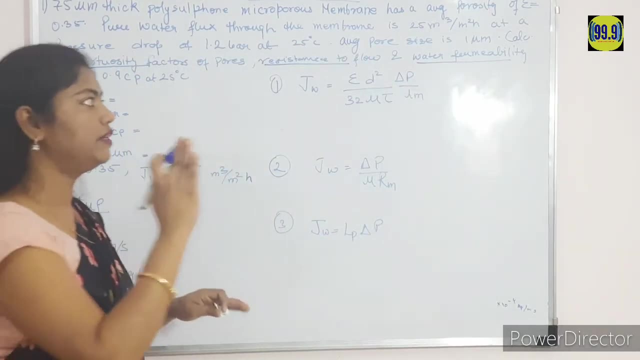 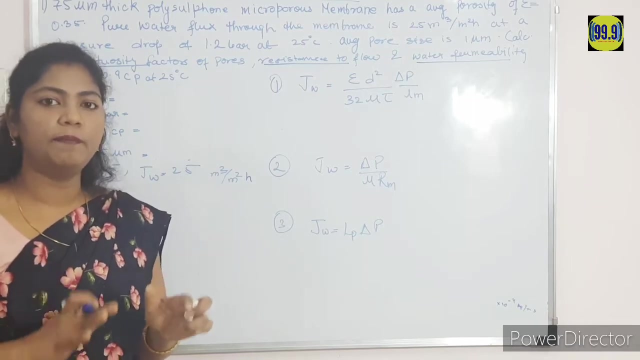 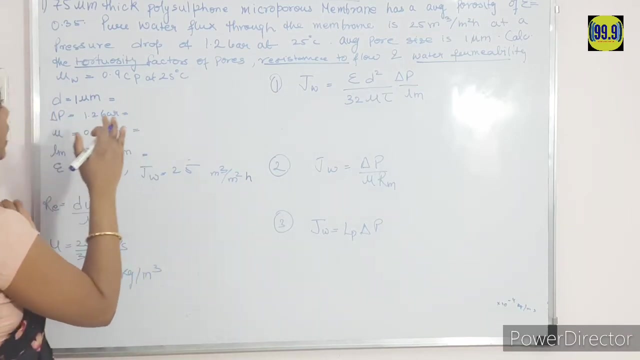 so we have to find out three things to calculate for the, that is, torricity factors, resistance to flow and water permeability. okay, so for cal, before going to calculating or write down the formula, first we write out the given parameter and convert into a proper unit. okay, so as as given in the given in the question, that average pore size is given. 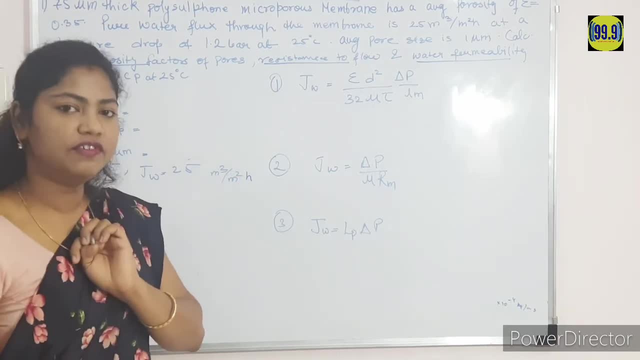 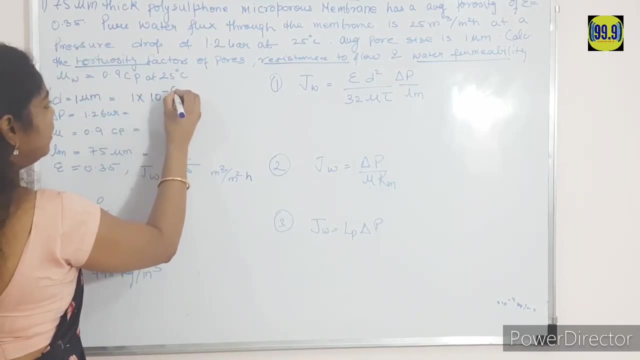 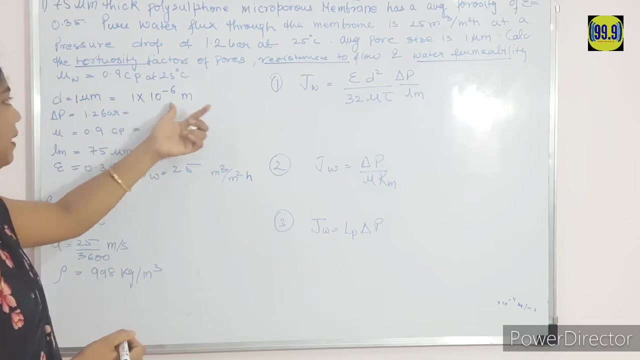 that is one micrometer. so we have to convert first one micrometer into a meter. so for converting it we simply multiply with a 10 to power minus 6, and then we get the average pore size in meter, that is 1, into 10 to power minus 6 meter. now another thing is given, that is pressure difference, that is 1.1. 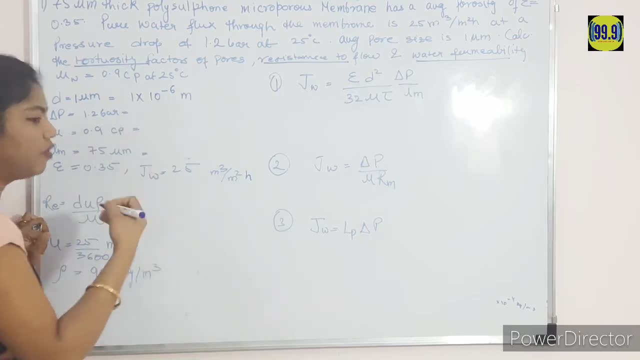 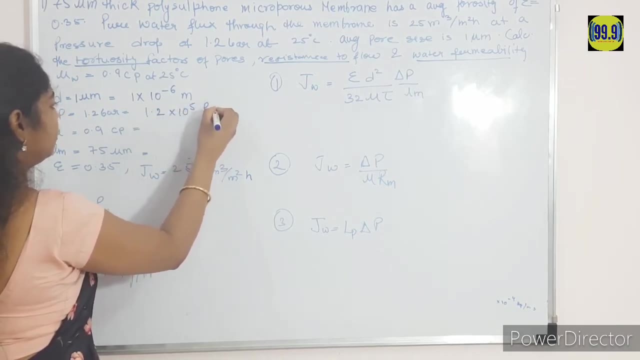 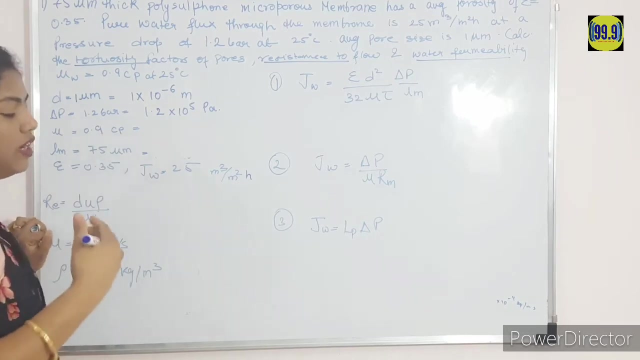 1.2 bar, so we have to convert into a pascal. for converting into a pascal, we simply multiply with a 10 to power 5 pascal, okay, okay. and another thing is a viscosity given that is 0.9 CP, so we have to convert into a kg per meter. second for: 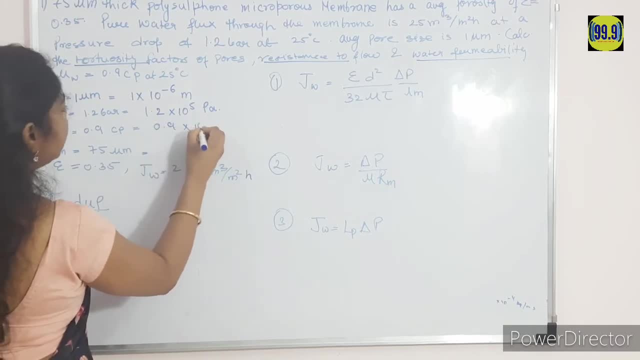 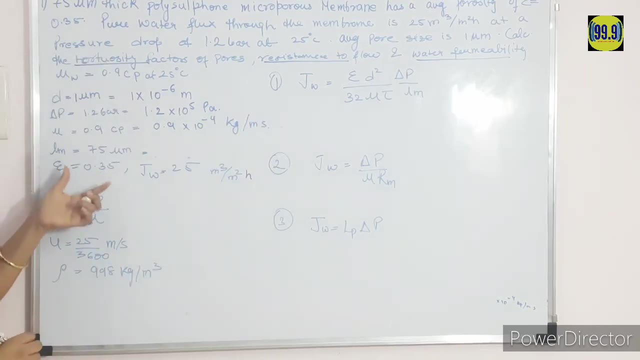 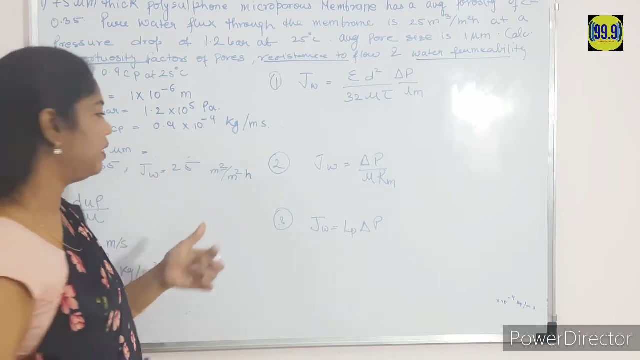 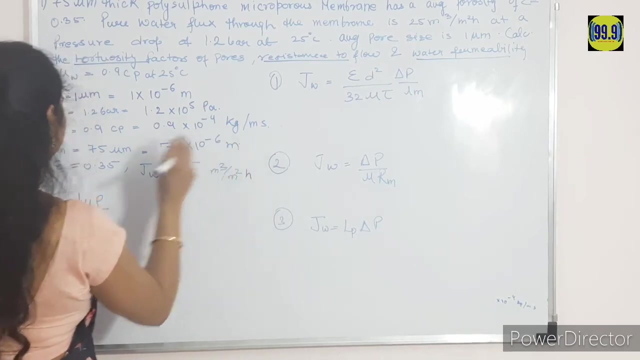 that we have to multiply it with 10 to power minus 4 kg per meter. second: okay, so another. another is: LM is: given the thickness of the membrane, it is given as 75 micrometer. so we simply multiply it with the 10 to power minus 6 meter. another data is: sigma is equal to 0.35. 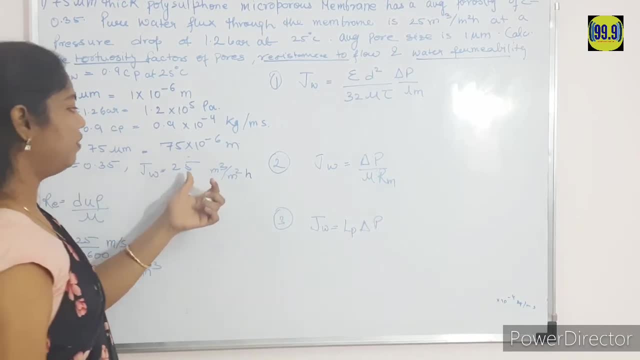 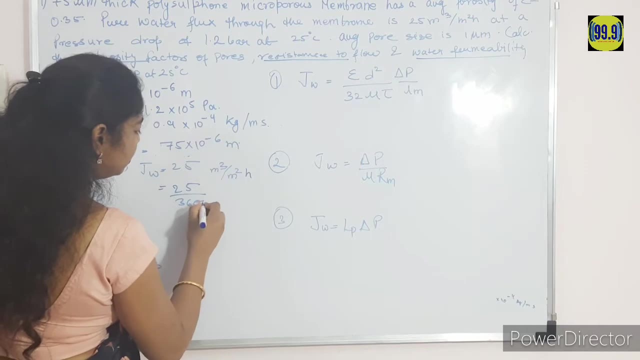 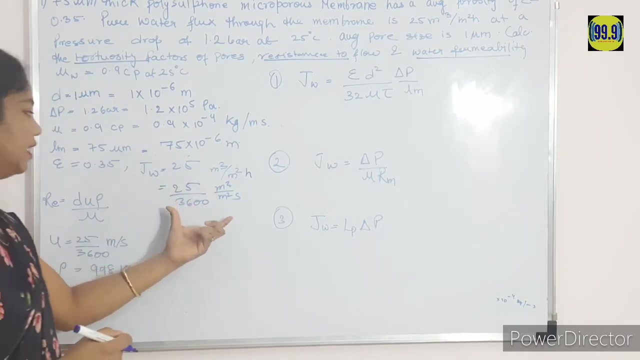 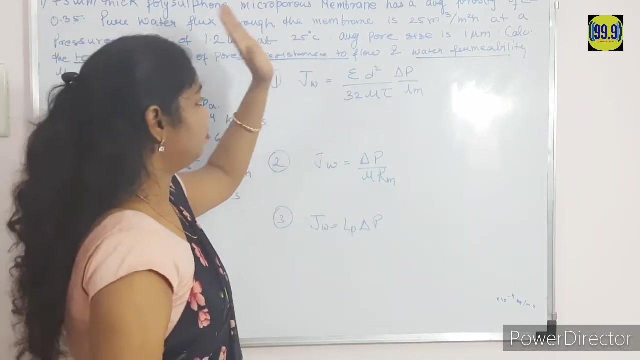 and jw flux is given, that is 25 meter cube per meter square per hour. so we have to convert into a 25 upon 3600 meter cube per meter square per second. okay, so flux is in this terms. so for calculating the first, for calculating the parameters, torticity factor, resistance flow, 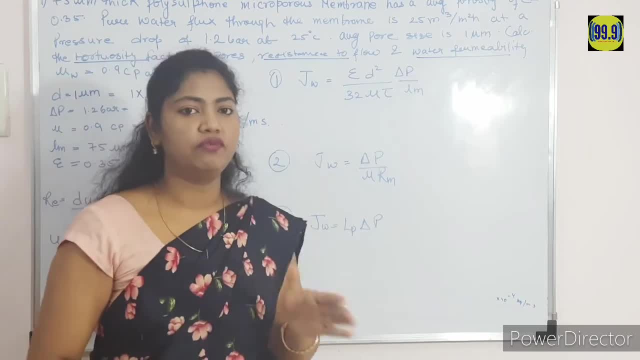 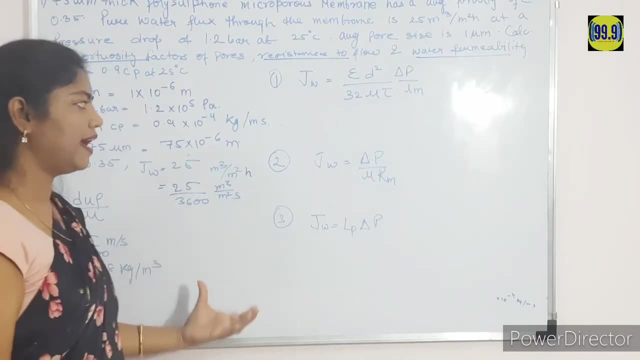 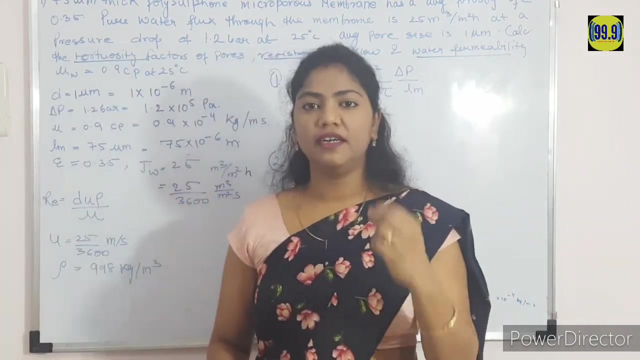 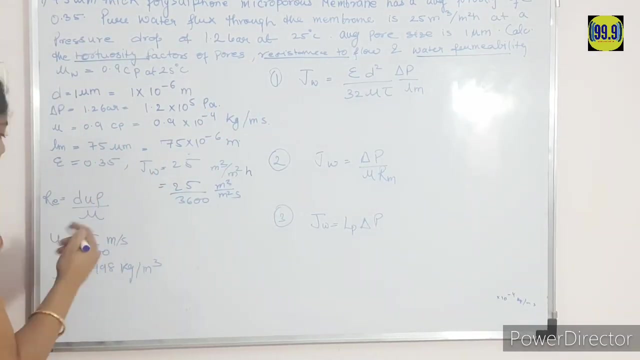 and the water permeability. first we have to check that the flow is laminar or another thing. so for calculating, calculating the laminarity, we need the form of what we need: viscosity, diameter, diameter, density and the velocity. okay, so the density, then viscosity is 25 upon a, viscosity is already. 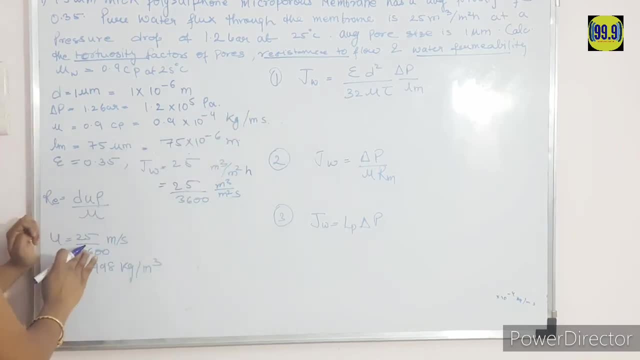 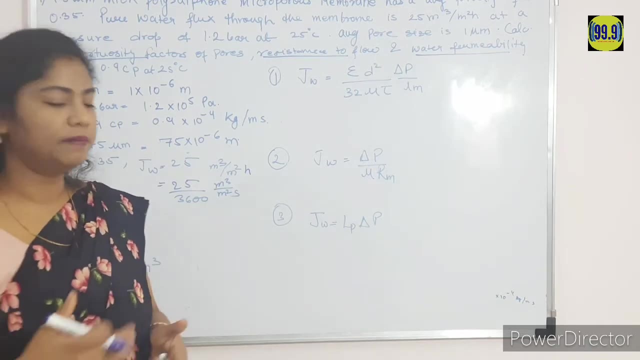 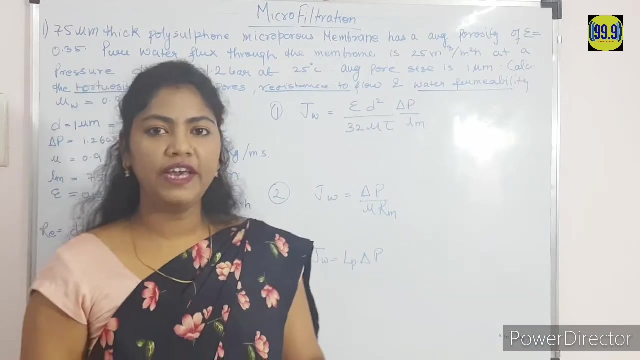 given that is 0.9 into 10 to power minus 4, and the velocity is calculated from this flux, that is 25 upon 366 600 meter per second, and the density of the water is 998 kg per meter. now we have all the data for calculating the renal number, so we have to simply put all the 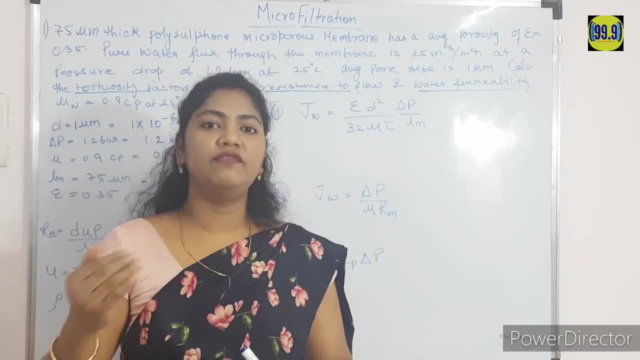 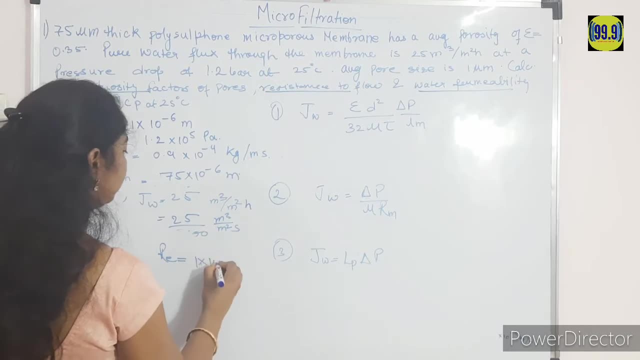 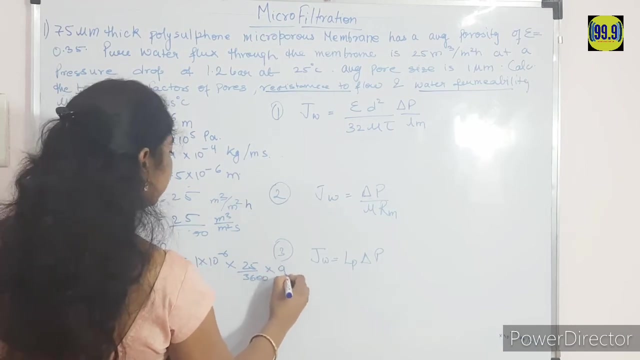 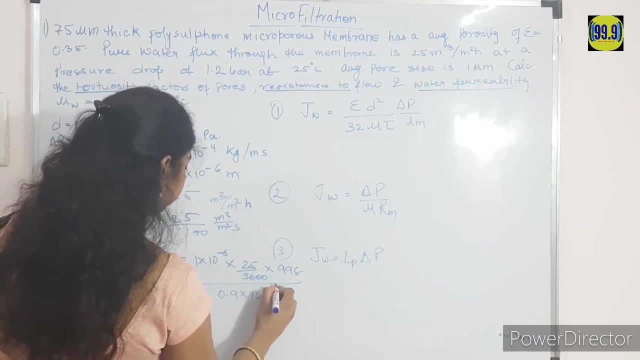 data in the renal number formula and then check that the flow is laminar or not. so let's do that. renal number is equal to d is given that 10 to power minus 6, u is us is 25 upon 3600 and the rho is 998 upon mu is 0.9, into 10 to power minus minus 4, and from here: 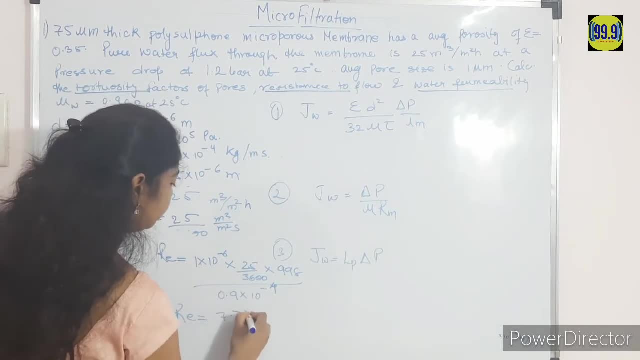 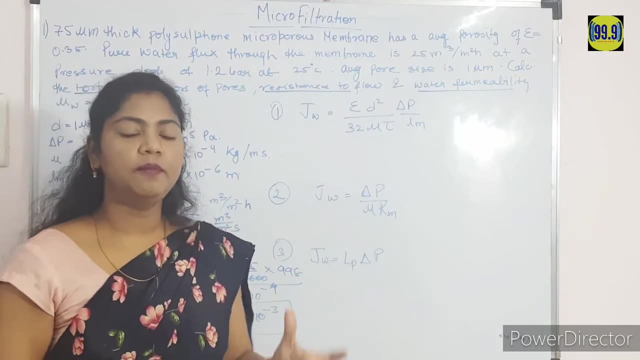 the renal number we get. that is 7.7 into 10 to power minus 3. okay, 7.7 into 10 to power minus 3, it means it is come under the range of laminar flow. it means definitely it is a laminar flow. 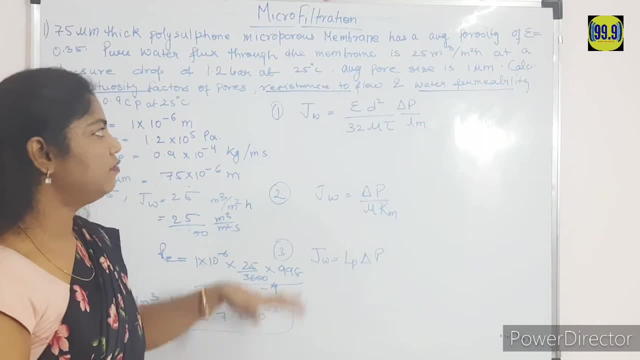 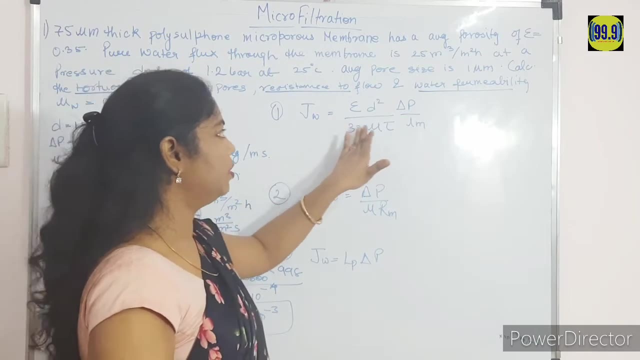 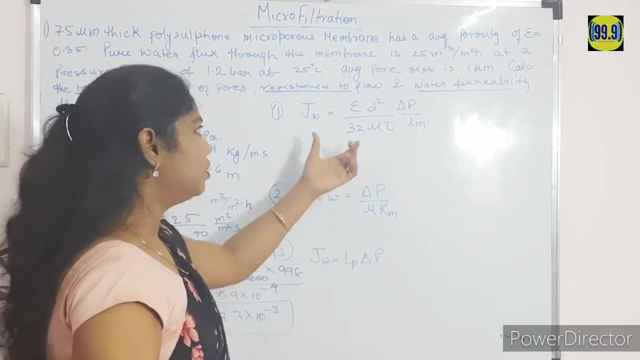 into a pore membrane. so it means we have to calculate the flux through the Heisen-Posley equation, which is a, which is equal to jw, is equal to sigma d square upon 32, mu, l, mu tor, delta p upon l m. so first we have to calculate the torticity factor. it means we have to: 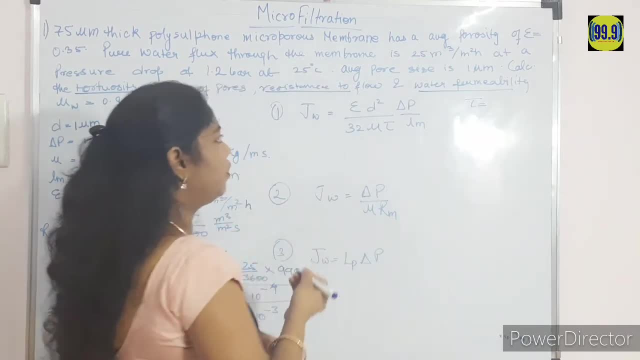 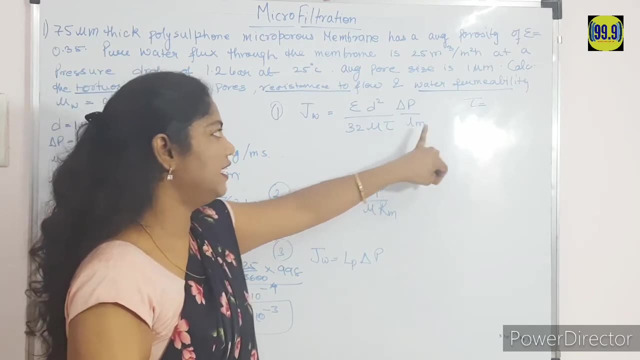 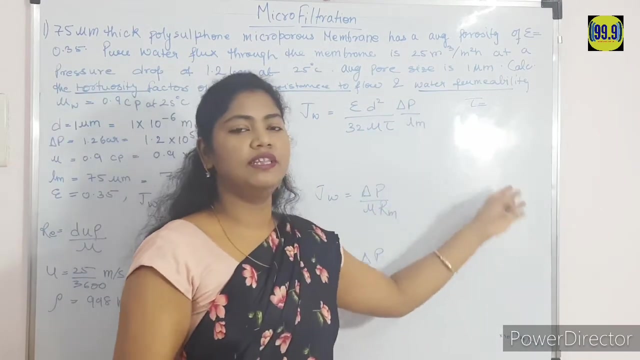 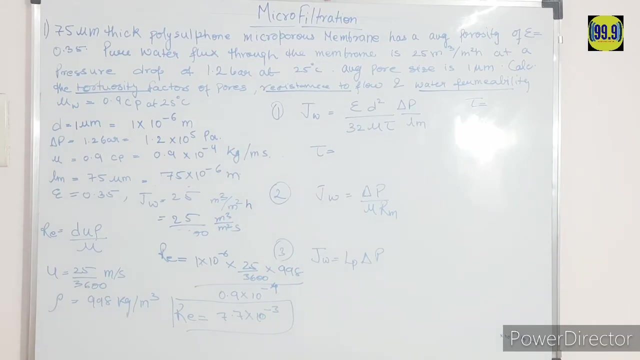 calculate the torp. okay, so just put all the values. we have a sigma value, d value, delta, p value, 32, viscosity in LM, all the value we have. we have GW value. so simply substitute all the value and we get from here. tor is equal to. we get from here: tor is equal to 2.8 torticity factor. we. 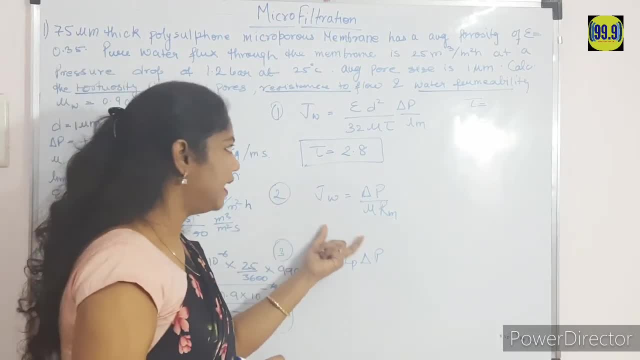 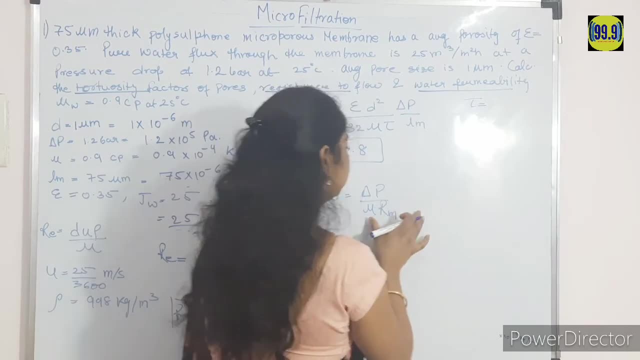 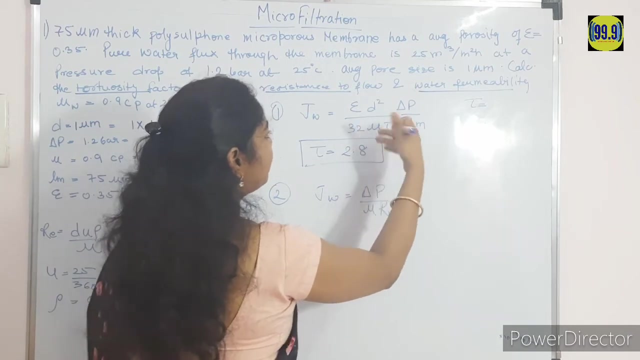 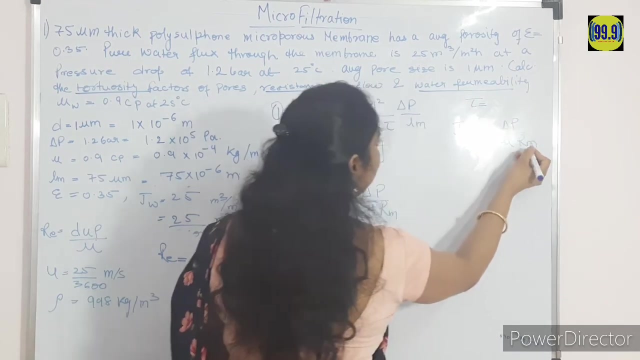 get from here. here, that is 2.8. next, we have to calculate the resistance of flow. for calculating the resistance for flow, we simplify this equation into a. this equation by: simplify this equation into a, which equation. we simplify this equation into a delta p upon mu rm, where rm is delta, rm is rm is which. 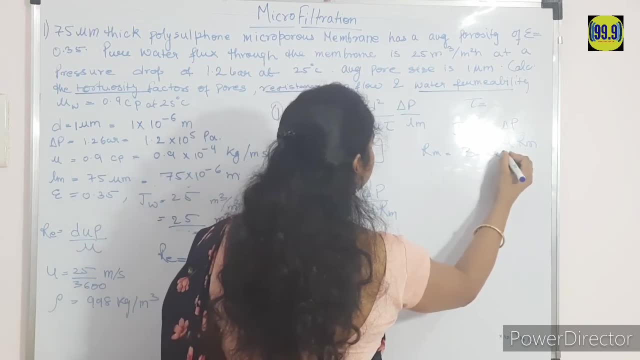 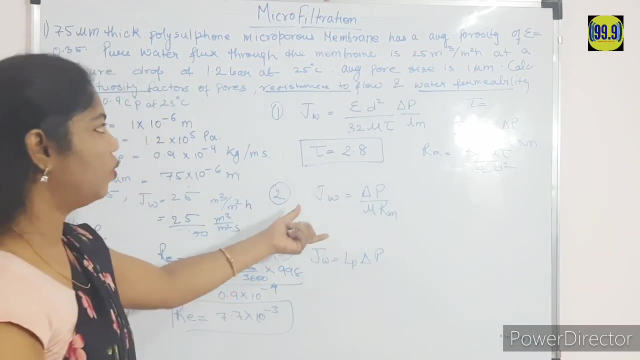 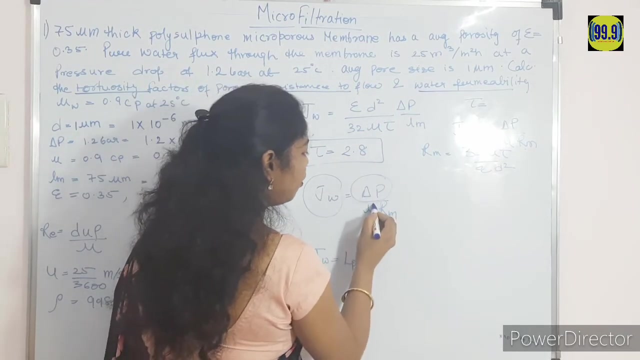 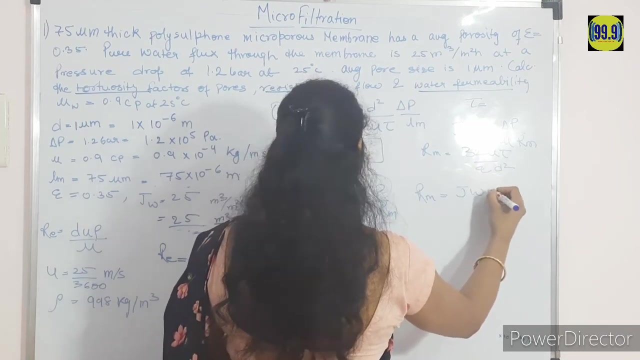 is sigma, is 32 mu tau upon sigma d, d square, this was, this was, and we have to calculate resistance. so how will we calculate? we know jw, we know delta p. now we also know the viscosity. we simply rearrange this equation like that into into mu upon delta p, and we get here from here.